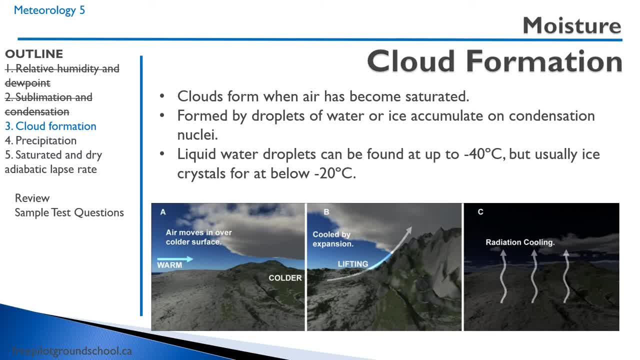 not form clouds. Clouds are formed when droplets of water or ice accumulate on condensation Nuclei, So there's another requirement for cloud formation is condensation nuclei. Liquid water droplets can be found at up to minus 40 degrees Celsius, but usually ice crystals. 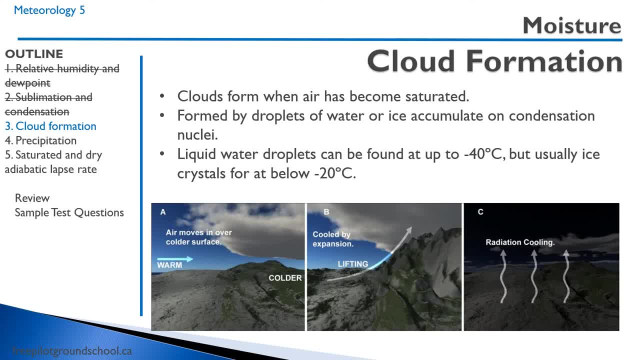 at below minus 20 degrees. So here's some examples of how we can end up with clouds. The first: we have warm, moist air moving over a colder surface. Remember, colder air holds less water vapor than warmer air, so the temperature will be cool to its dew point. 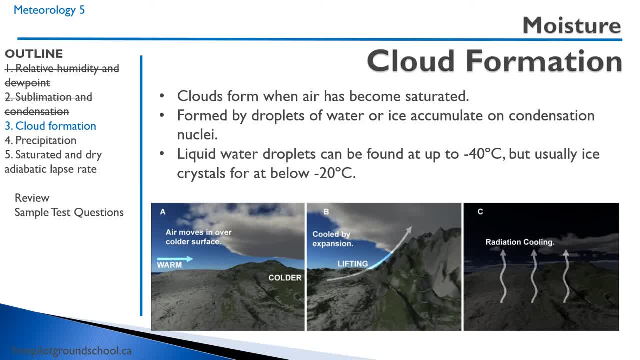 As it moves there to the dewpoint, the air becomes saturated and the water vapor condenses into water droplets. Secondly, in panel B, there we can look at, the air is cooled by expansion. If we force air up the side of the mountain as we, the air goes up. it will expand, As it expands, it will cool and as it cools. 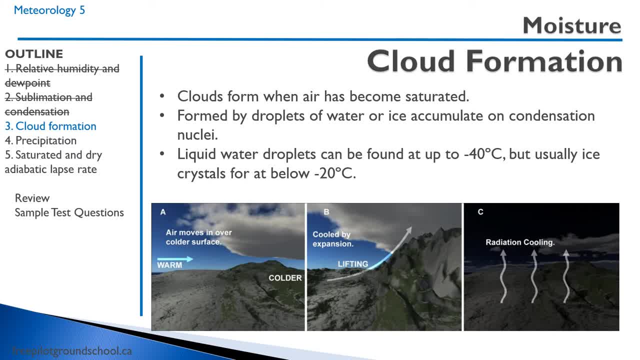 eventually becomes saturated and the water vapor will become water droplets. Last point: we can have radiation cooling. this is when we have radiation fog, the warm, moist air over the earth. at night time the earth loses its uh heat to uh radiation into space. the temperature of the air. 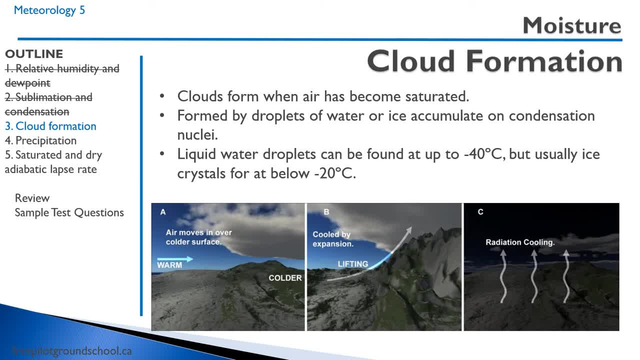 cools to the dew point, find this often uh, cold, clear nights. let's just say, take a look at the temperature. dew points break. you might say, oh look, this looks like a beautiful night for flying, but you don't realize that very quickly you might end up with very thick radiation fog. 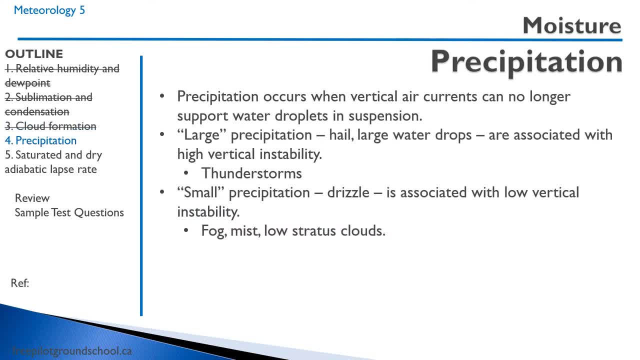 precipitation occurs when vertical air currents can no longer support water droplets and suspension, so sometimes you'll notice that the precipitation is large. we have large hail, large water drops. you're outside, it starts raining and it's really pouring down hard and that's associated with high 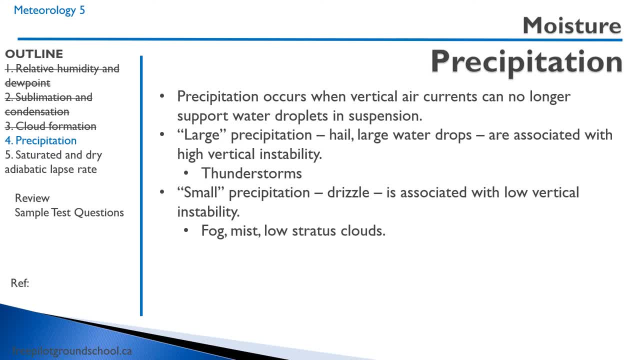 air pressure and that's associated with high air pressure and that's associated with high vertical instability, such as thunderstorms. so the water droplets uh form and then with air currents they get pushed back up, where they cool us with more water droplets and they get. 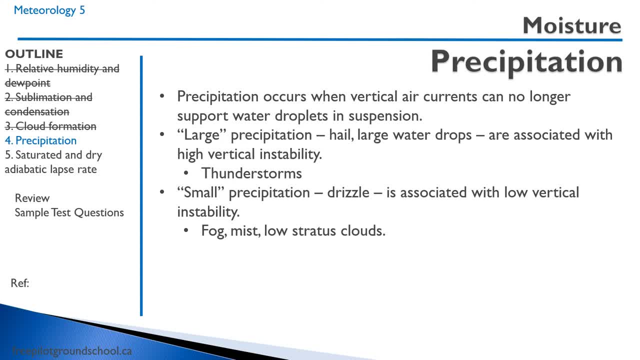 larger and larger and larger until they're so heavy that the vertical updrafts can no longer sustain them. that's how we ended up with very large hail just keeps building and building and keeps getting blasted back into the top of the thunderstorm and creating more. 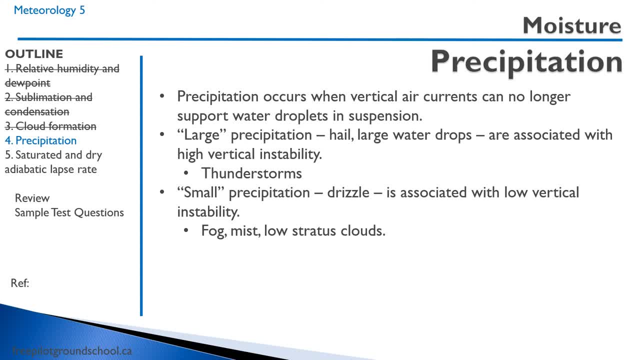 and more and more ice on it. then you have small like small precipitation, like drizzle, associated with low vertical instabilities from stratus clouds. you end up with fog, mist and low stratus clouds. it's very stable. there's no vertical updrafts to keep that. those water droplets in the 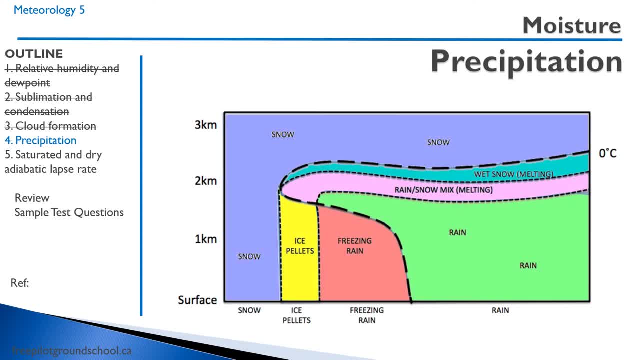 air, the chart on how we have different types of precipitation, with altitude, so, for example, we can have snow from the surface up into high altitude. on the opposite side, we have rain down low and then, when we have inversions, we end up with things like freezing rain. so you look for. 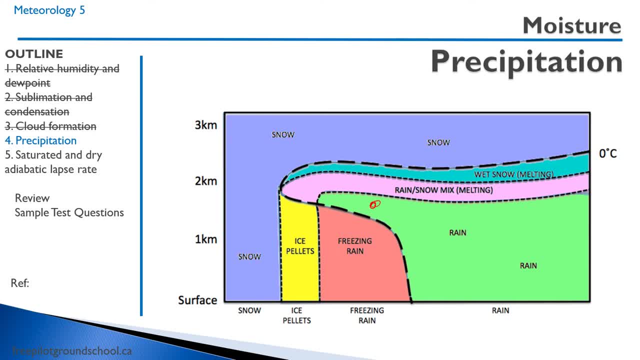 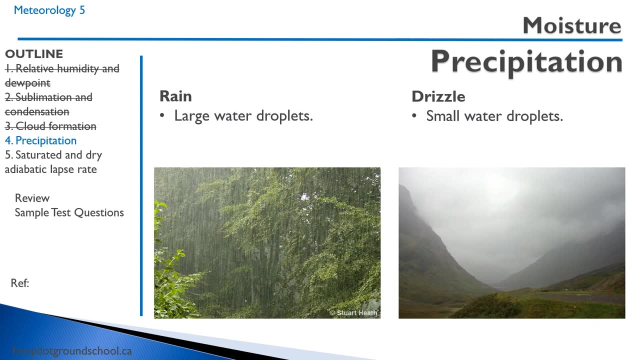 example, right here. okay, the rain falls, it's cooler down here and then, as it hits the ground, it ends up freezing. same thing with ice pellets. here you can have that. you can have a lot of different types of precipitation. rain is large water droplets on the left and drizzle small water droplets on the right. snow are crystals of frozen water. 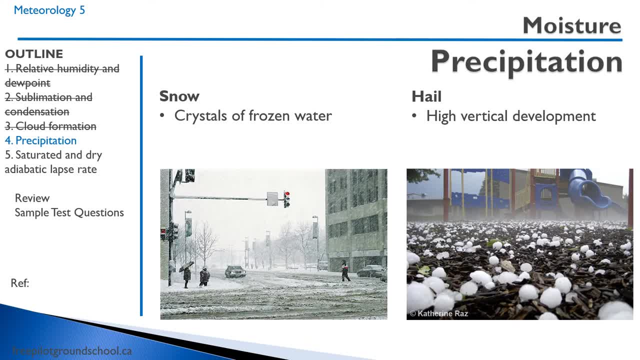 and obviously everyone knows what snow is like if you live in canada. i think this is from winnipeg. looks like winnipeg anyway. on the right we have examples of hail. they're kind of chunks of ice and they're associated with high vertical development, which is 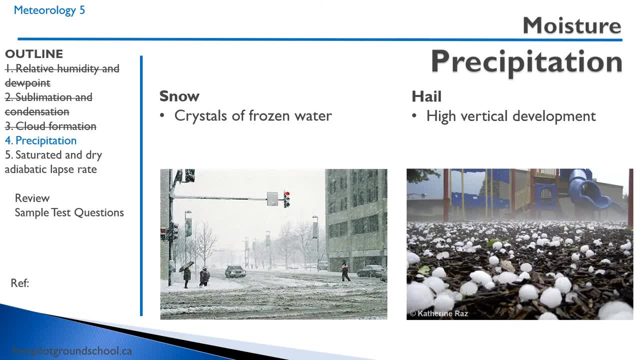 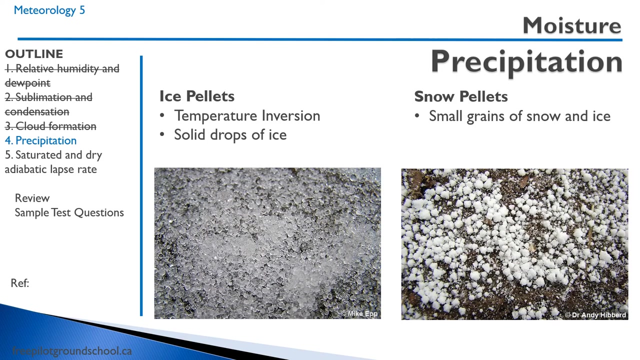 thunderstorms, where precipitation is forced high into the tops of the clouds, where it picks up additional snow and ice falls back down and gets blasted back up again and keeps. basically very hard ice snowballs keep forming on this and getting bigger. next we have ice pellets, and ice pellets are distinct from hail. like we said, hail is from unstable air, cumulonimbus clouds. 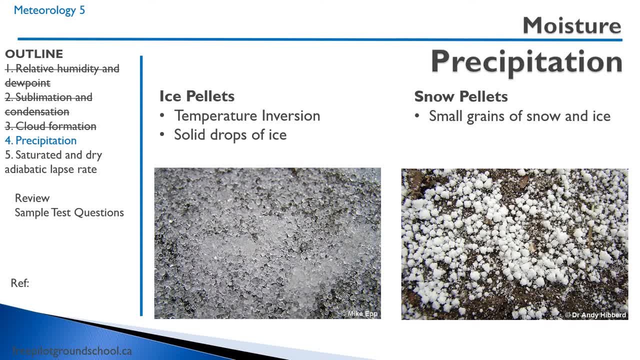 and the ice pellets are caused by a temperature inversion. we have rain at altitude and at lower altitudes we have uh colder air. that rain falls into the colder air and freezes on its way down and they're just frozen solid drops of ice. if uh snow pellets, it's a kind of a hybrid. they're small. 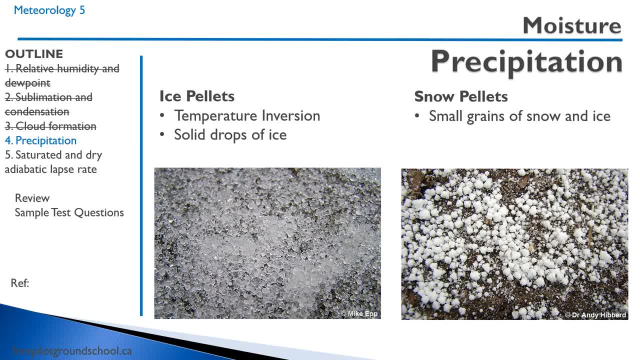 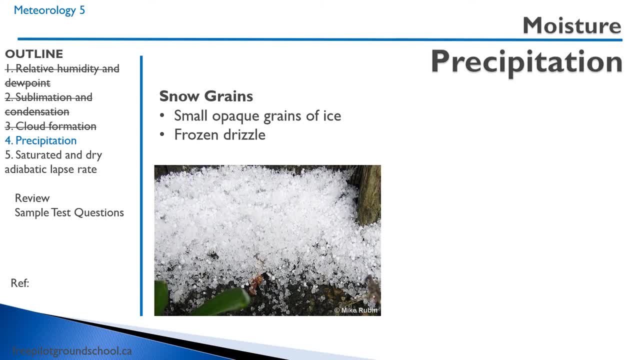 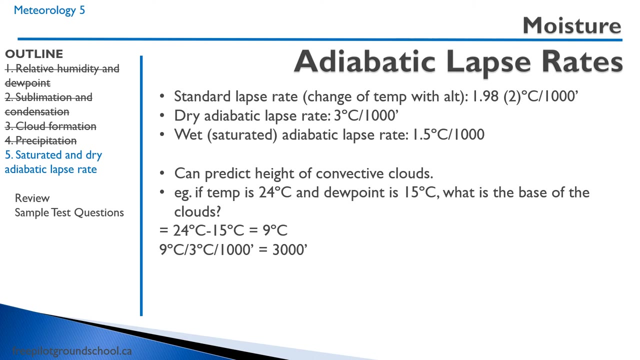 grains of snow and ice. lastly, we'll talk about snow grains. these are small, opaque grains of ice and they are frozen crops drizzle. So just like you have ice pellets, these are, when you have drizzle, freezing up. Touched on this. the last lesson: the adiabatic lapse rates. We have a it's roughly two degrees. 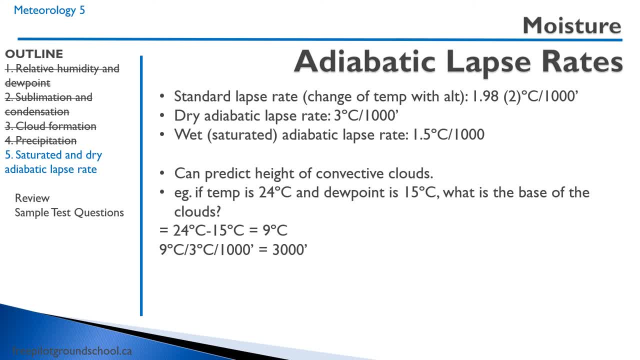 per thousand feet on average, but when it's dry it's three degrees per thousand feet, And when it's wet it's 1.5 degrees Celsius per thousand feet. We can predict the height of convective clouds as well as the freezing level. which point? at what altitude does the atmosphere freeze? So 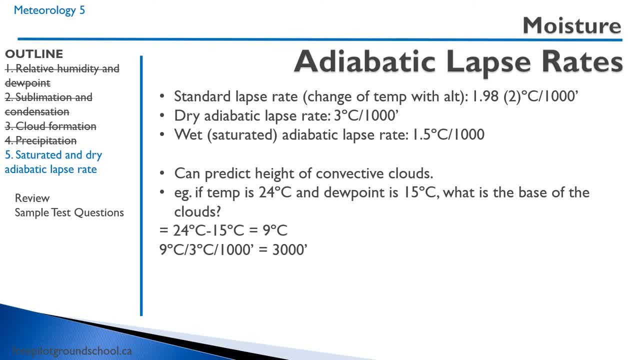 here's an example: Temperature is 24 degrees and a dew point 15 at the base of the cloud. So 24 minus 15 is a nine degree spread, because it's dry below the clouds. three degrees a thousand feet. So nine degrees divided by three 3,000 feet. Dew point is the temperature to which a volume of air at 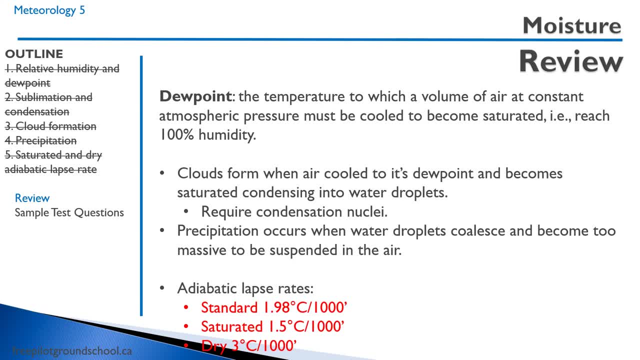 constant atmosphere. Dark pressure must be cooled to become saturated, So reach 100% humidity. Clouds form when air is cooled to its dew point and become saturated, condensing into water droplets, And these clouds require condensation nuclei. Precipitation occurs when water droplets coalesce and become too massive. 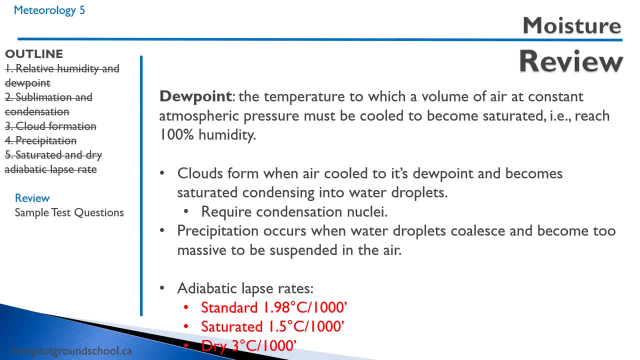 to be suspended in the air. The standard lapse rates are 1.9 to 8 degrees Celsius per thousand feet Saturated. so when it's wet it's 1.5 degrees Celsius per thousand feet and dry is three degrees Celsius per thousand feet. 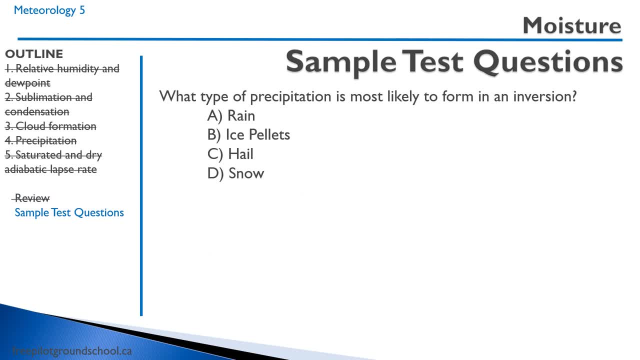 What type of precipitation is most likely to form in an inversion? So remember, an inversion is when the temperature increases with altitude, So up high it'd be warm. so let's say you have rain and then the ice or, I'm sorry, the rain falls into. 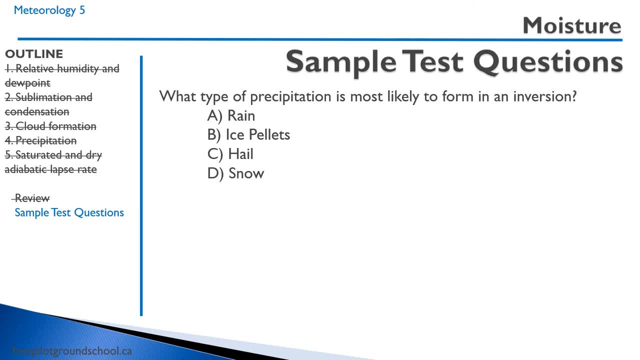 colder air below. So let's go through these. a rain, no, that's just, it would stay as uh, rain um ice pellet. So this is the correct answer, or here is ice pellets. so if we recall, uh, if we draw a line here and it's raining here, 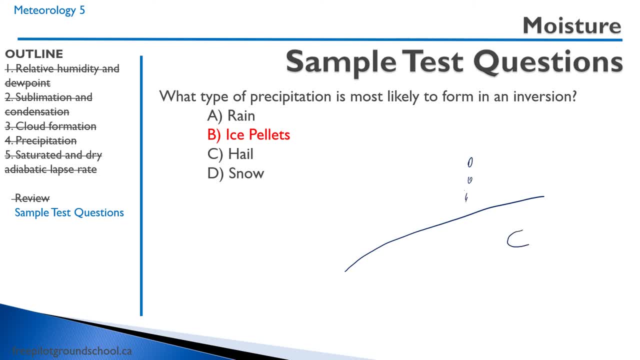 it's raining and now all of a sudden it's cold, cold and hot, okay, and then it comes here and then, all of a sudden, it starts cooling, cooling down and hitting the ground as solid chunks of ice. so hail is not correct because, remember, hail is not from an inversion, it's from. 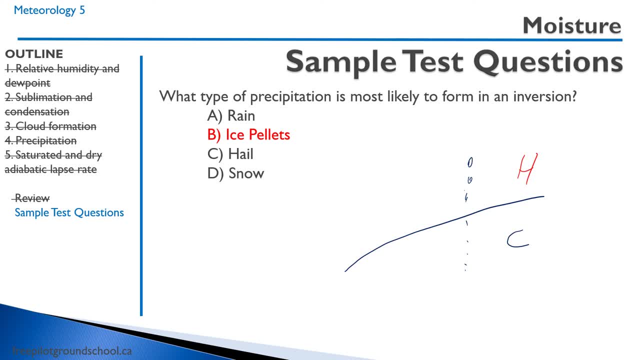 thunderstorms and unstable air and snow is not correct either. what type of precipitation is most likely to form when there is extensive vertical instability? so we kind of briefly touched on this last question. the correct answer is going to be hail. so remember what happens with hail: the precipitation falls and then gets brought back up. 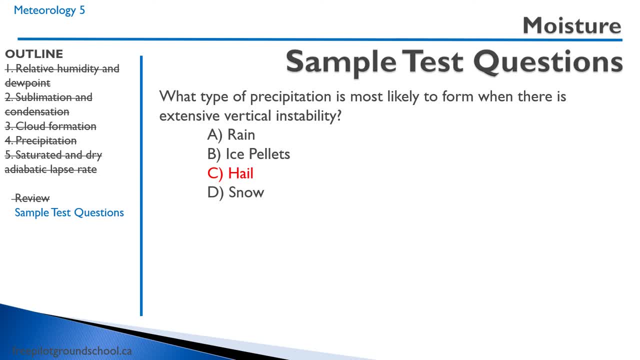 from the vertical updrafts, at which point more moisture is accreted on to the existing hail particles and the more instability. the more updrafts we have, the larger hail we end up getting. what conditions do not need to be present for clouds to form, so a our water vapor. so recall we. 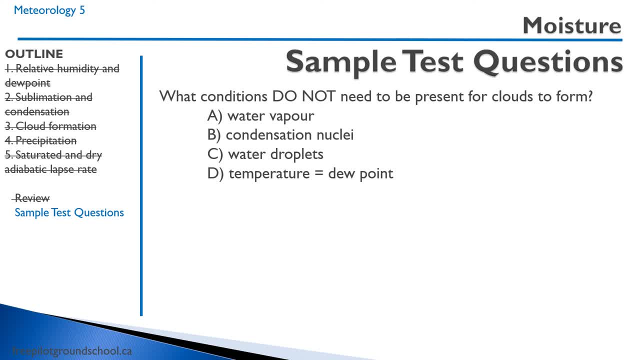 do need water vapor for class form b condensation nuclei. so we need condensation nuclei. we need for that water vapor to condense onto c water droplets. well, no, that's not correct. we don't need water droplets for clouds to form. clouds form and you get water droplets. d temperature: 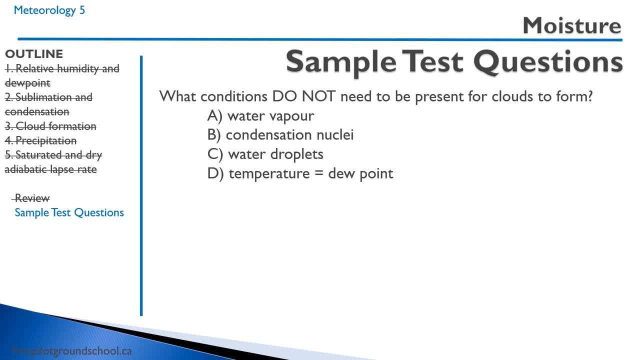 equal dew point. yeah, the air has to be saturated for the water vapor to condense into- uh, water droplets. the correct answer is c- water droplets. so here's a question that, uh, we'll see if you can remember how to do, because you're very likely to get it on your test.